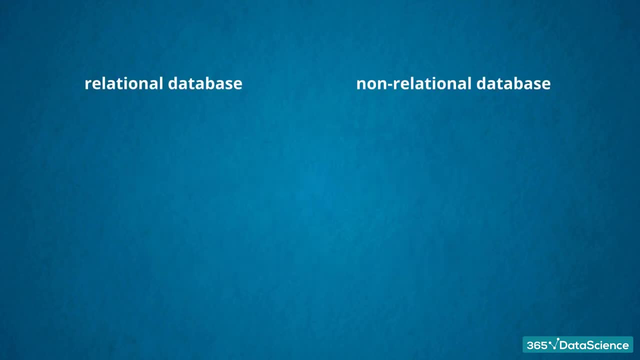 You should remember, there are two main types of databases: relational and non-relational. The former will be the focus of this course, while the latter regards more complex systems. Although understanding non-relational databases requires a serious mathematical and programming background, some of the logic applied in its coding is the same as SQL. 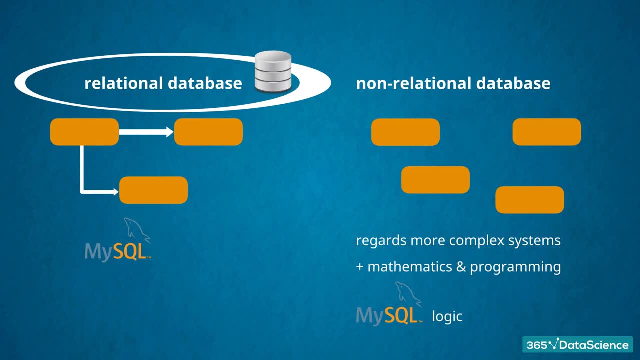 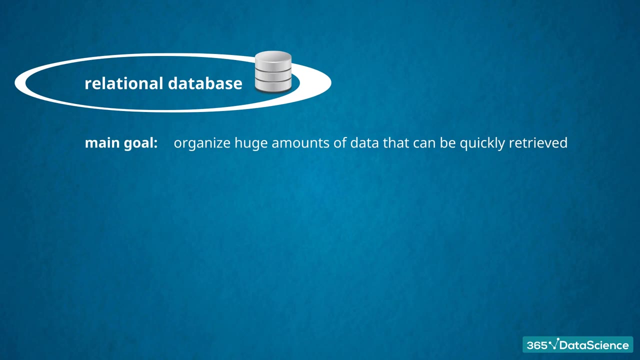 Likewise, relational databases have a few advantages on their own. A small bit of theory will explain why they are still the preferred choice in many companies and institutions. Databases' main goal is to organize huge amounts of data that can be quickly retrieved upon user's request. 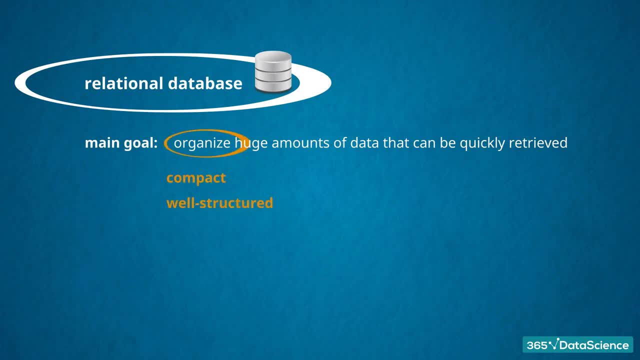 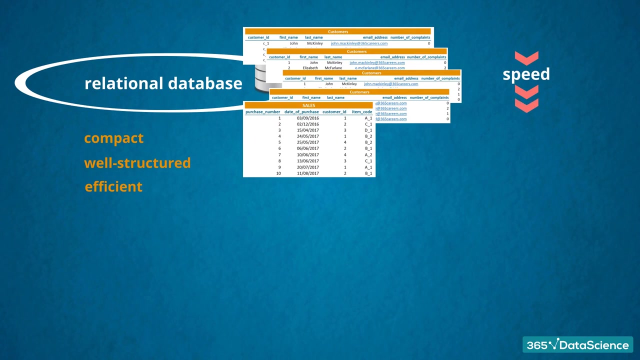 Therefore, they must be compact, well-structured and efficient in terms of speed and data extraction. Today, people need such extra efficiency because data occupies memory space and the bigger its size, the more sluggish the database is and the slower the retrieval process becomes. 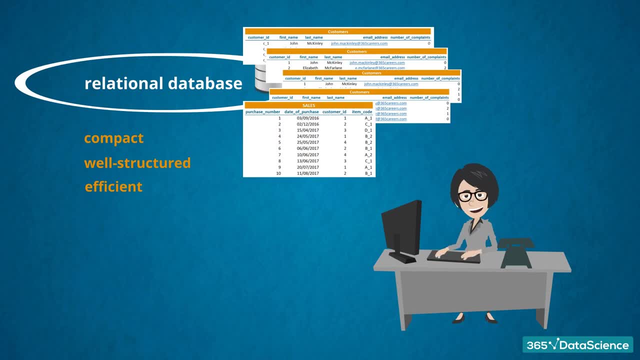 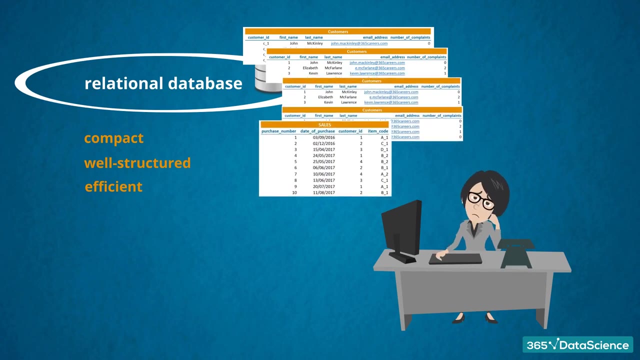 If we have a database containing one multi-million row table with many columns, then every time a request has been received, the server must load all the records with all fields and it would take too much time for a task to be completed. Don't forget: every symbol is a container of information and requires bytes of storage space. 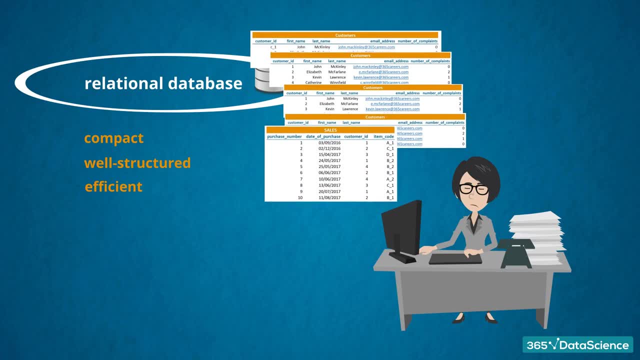 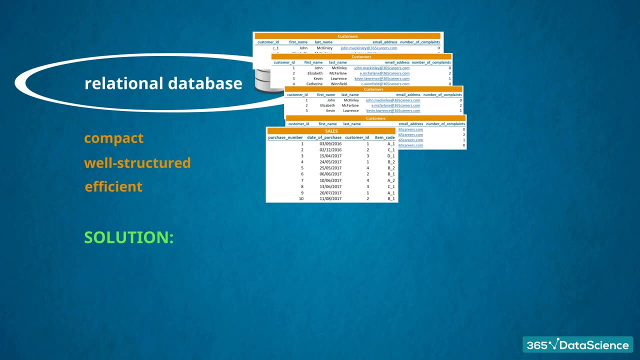 Hence, loading that much data will not be an easy job for the computer. So what allows us to contain so much data on the server, but lets us efficiently use only the portions we need for our analysis? The secret lies behind the use of mathematical logic. 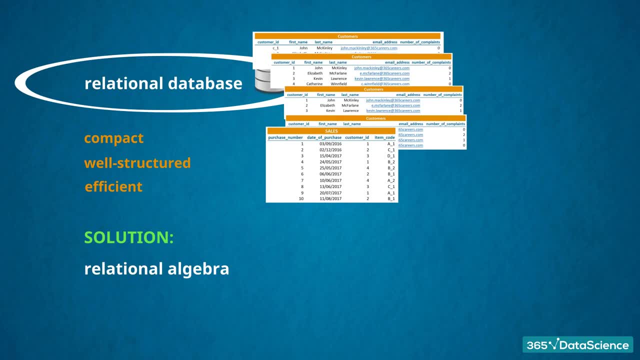 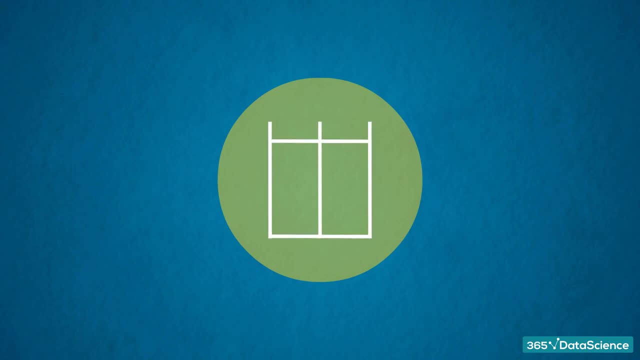 originating from relational algebra. Please don't worry, we will not bother you with math. Imagine: each table with data is represented by a transparent circle that contains all the data values of the table, categorized by columns or, as we will often call them, fields. 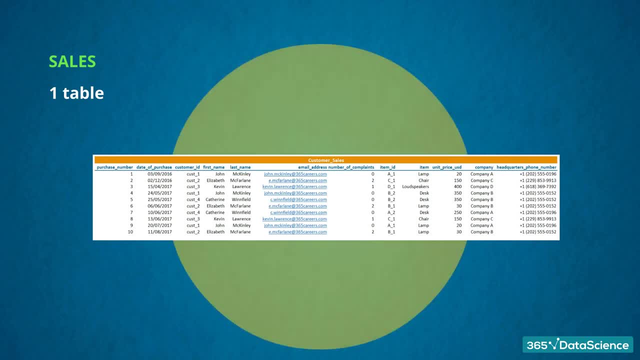 Now, if our database consisted of only one table, a giant circle would represent the entire database, something like this huge table from our fictional example with the cell's database. And when we need a piece of information, for example if we wish to see who has bought something on a certain date. 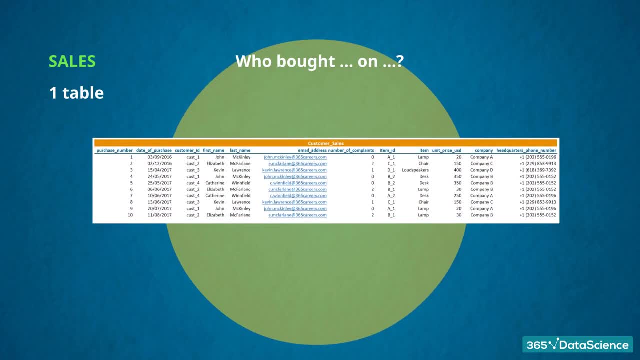 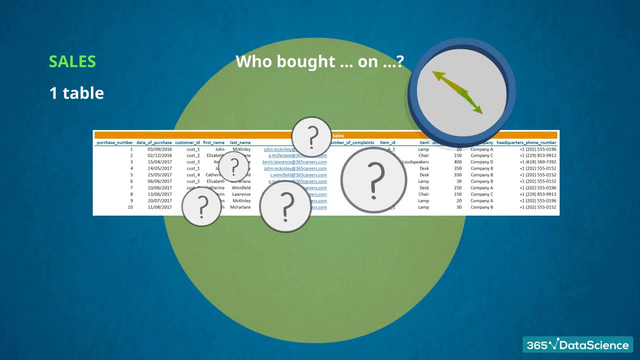 we will have to lift the whole big circle and then search for what we need. This challenge seems vague and the process of data extraction will not be efficient. See what can happen if we split the circle into three smaller circles, just as we did with the cell's database. 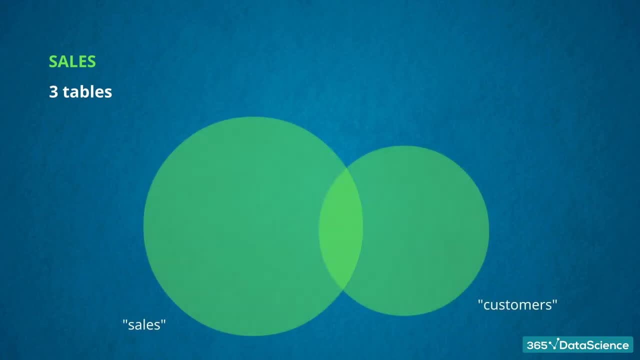 One circle will stand for the cell's table, the other for customers and the last one for items. There are various theoretical combinations between three or more circles, but in our database we have the following model: Cells and customers have the same customer ID column. 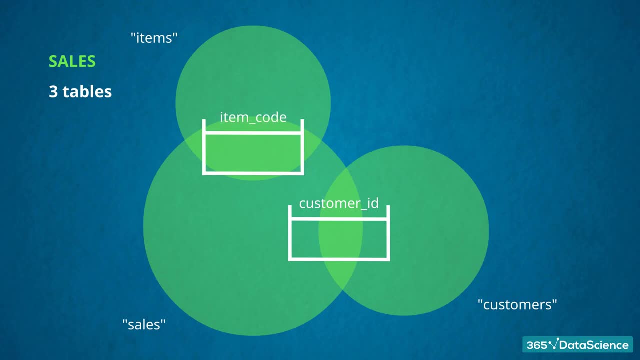 and cells and items have the same item code column. This way we can see the circles overlap as they have common fields. So if we'd like to extract the same information- the name of the customers who have purchased something on a given date- 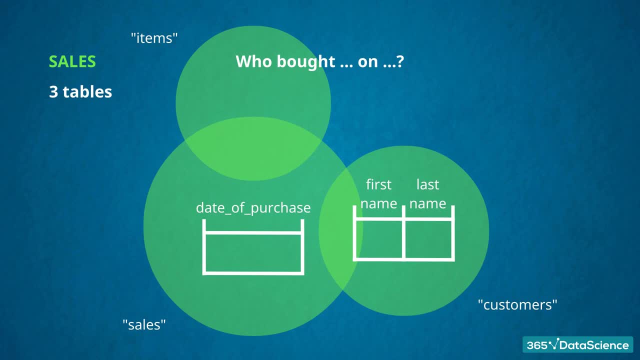 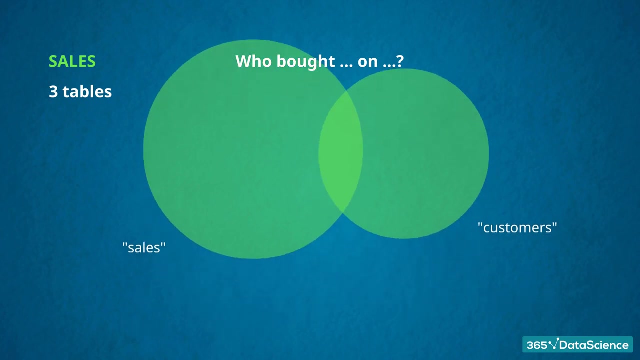 we will need only the date of purchase column from the sales table and the first and last name from the customers table. So to satisfy this request we will not need to lift the third circle from our database items. This way we can save energy or, more technically, increase efficiency. 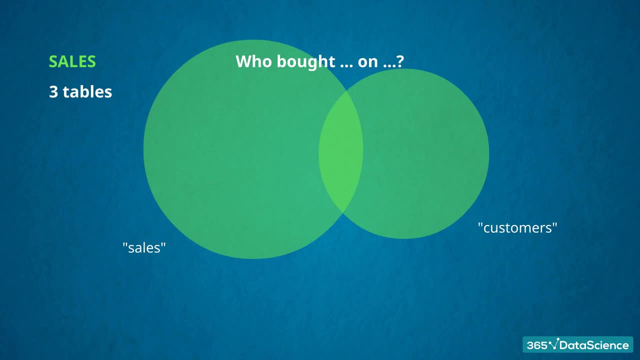 Less data represented, as only two of the three circles will be involved in this operation. The mathematical trick lies in relating the tables to one another. Relationships were formed mainly through these common fields. More explanations about this technique will be provided in our next lectures. 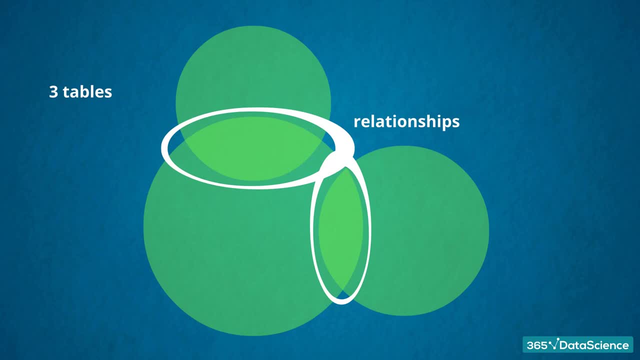 Anyway, I am sure that now you understand why we use the term relational databases. Some professionals may refer to the tables or the circles in our plot as relations because theoretically they are the smallest units in the entire system that can carry integral logical meaning. 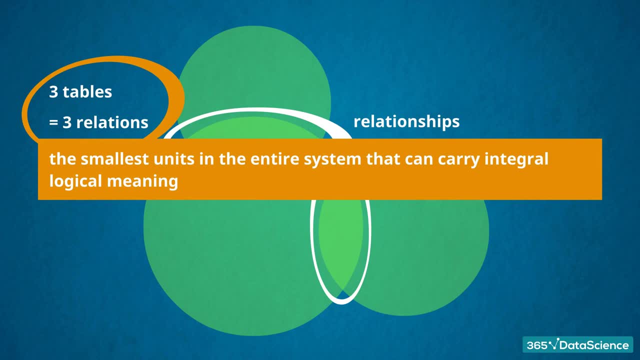 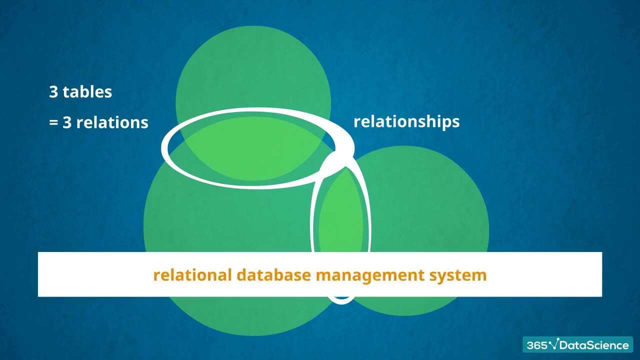 Likewise, the three circles are all part of our cells database. When we combine the database and its existing relations, we obtain the famous term relational database management system, frequently abbreviated as RDBMS. We hope this theoretical illustration makes things clearer. SQL is designed for managing relational database management systems. 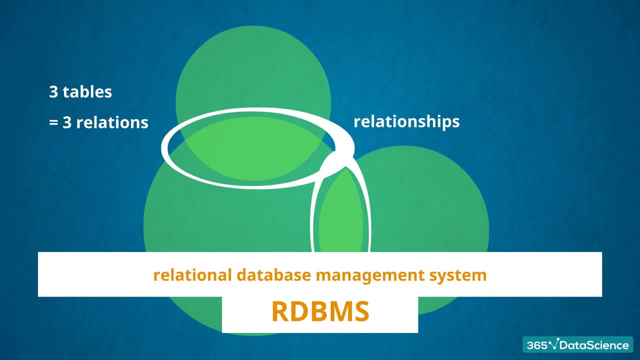 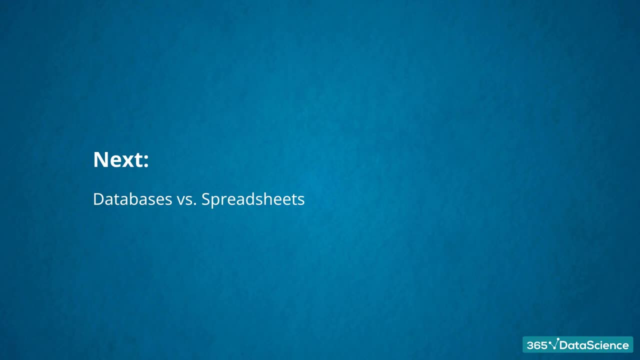 and can do that by creating relations between the different tables in a database. Stay tuned for the next lecture, where we will outline the most substantial differences between a database and a spreadsheet. Thank you for watching, Subtitles by the Amaraorg community.